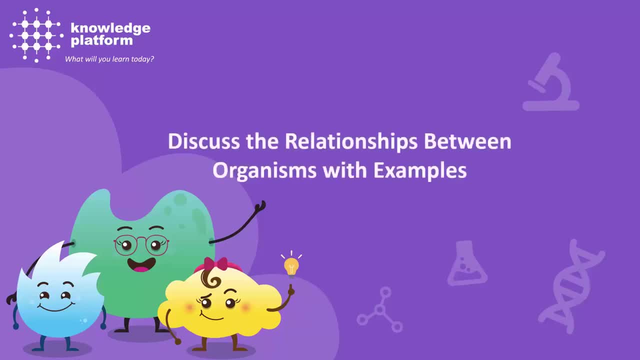 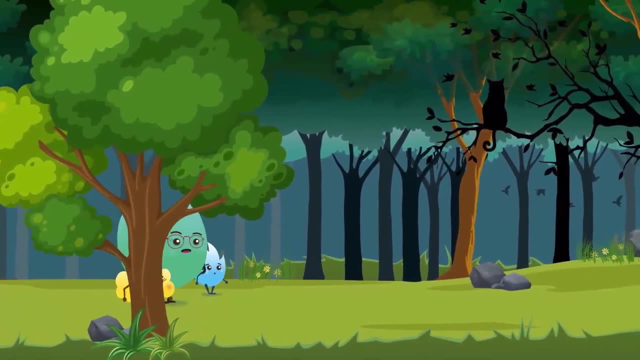 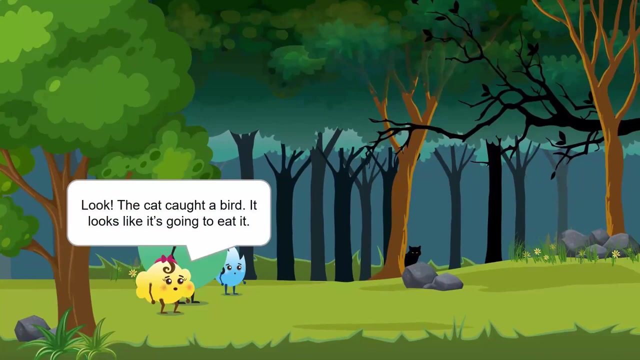 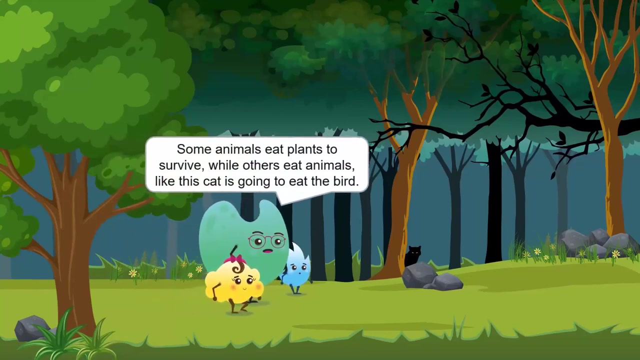 MrsCoco, look, The cat got a bird. It looks like it's going to eat it. Yes, Bubbles, Living things depend on one another for food. Some animals eat plants to survive, while others eat animals, Like this cat is going to eat the bird. 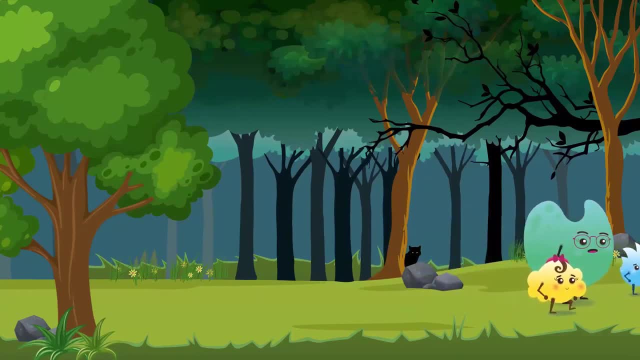 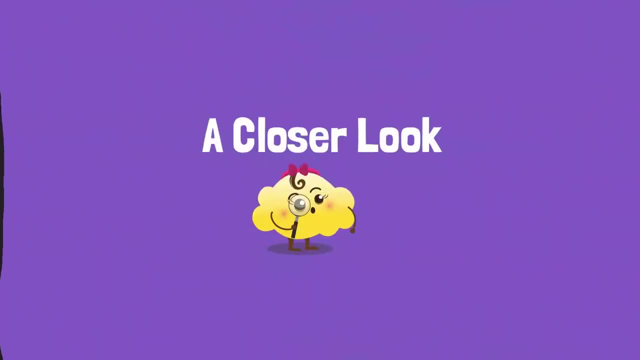 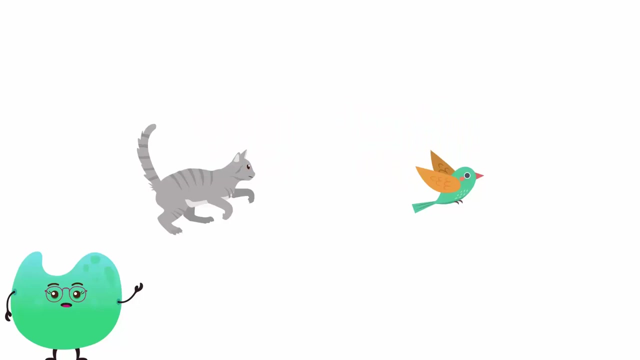 Different organisms depend on each other in different ways. Let's take a closer look at these relationships. For example, let's look at the cat and bird. In this process, the cat is a predator. A predator is an organism that kills and eats another organism. 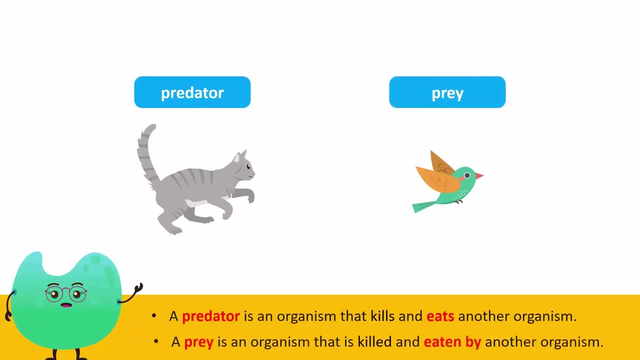 The bird was the organism that was killed, so it is the prey. Oh, must a predator always be an animal? And what about the prey? Good question. Both predator and prey can be either animals or plants. For example, if a goat eats a plant and the plant is unable to grow again. 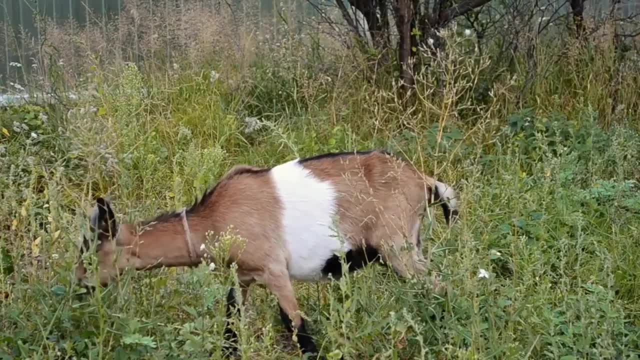 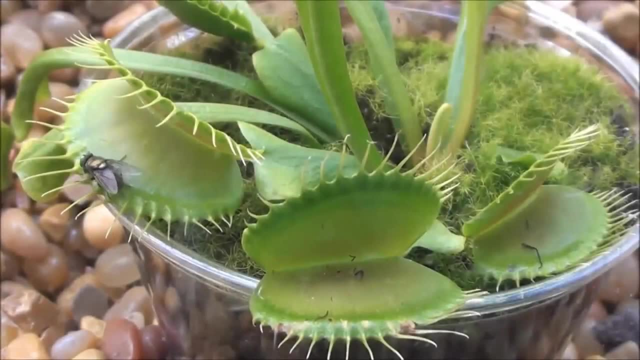 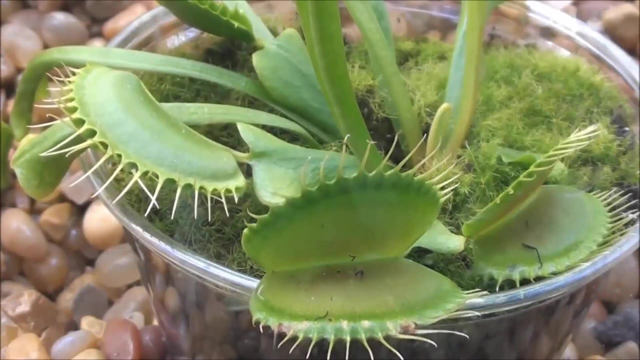 since its reproductive parts are eaten. that would make the plant a prey and the goat a predator. The flytrap is a plant that feeds on insects. It attracts insects through its color and nectar. Once the insects land on its leaves, it traps them and slowly digests them. 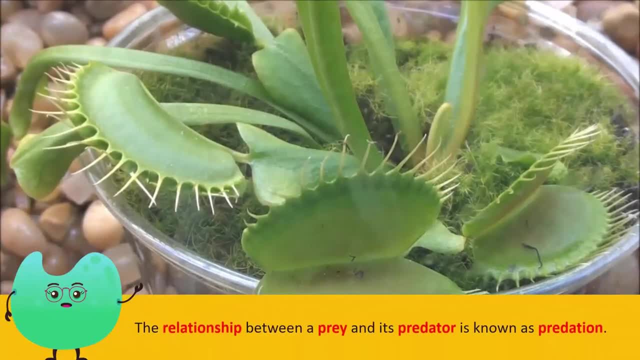 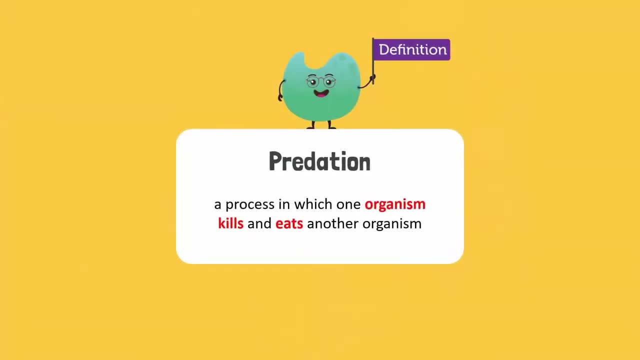 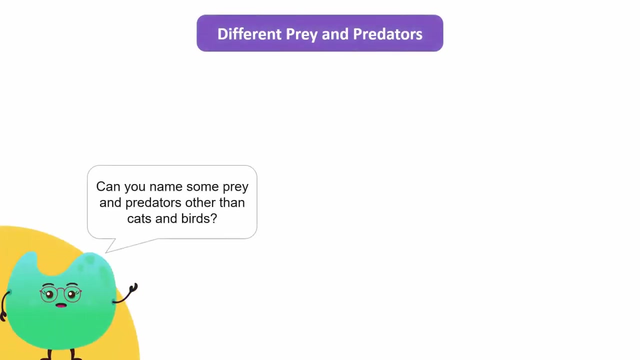 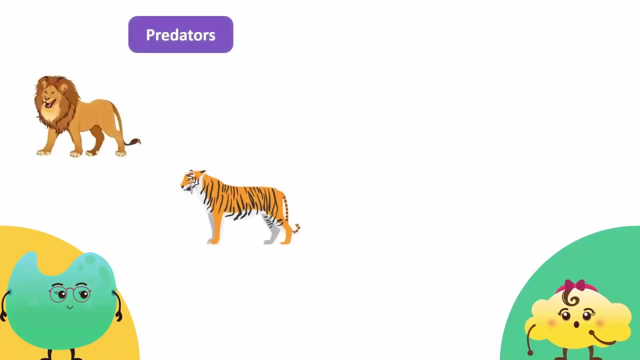 This relationship between a predator and its prey is known as predation. So predation is a process in which one organism kills and eats another organism. Can you name a few preys and predators other than cats and birds? Lions and tigers are predators that eat goats, deer and zebras. 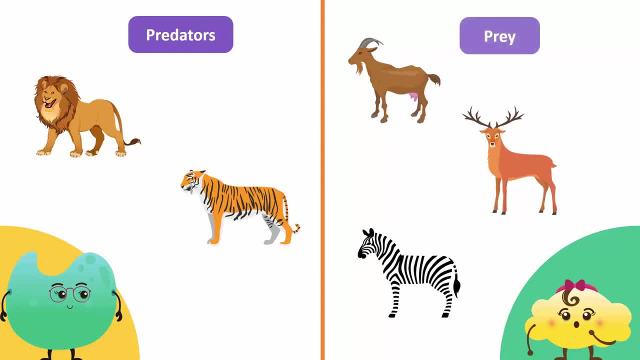 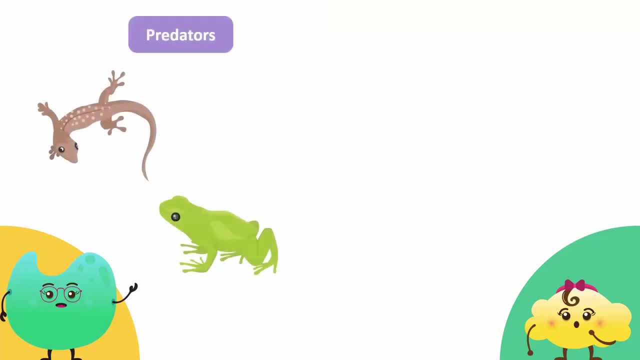 So goats, deer and zebras are prey. Well done, Bubbles. Subtitles by Subtitle Workshop. Lizards and frogs are predators as well for insects like flies, grasshoppers and mosquitos. Ah, I hate mosquitos. It hurts when they bite me. 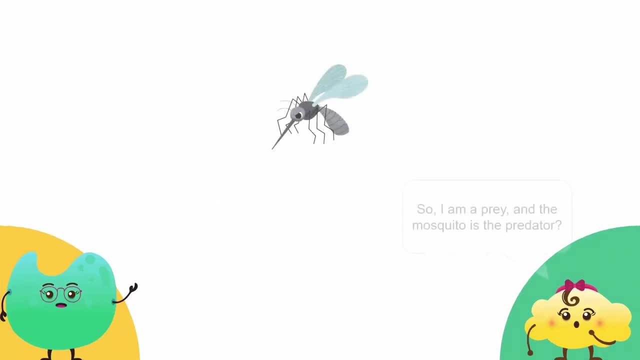 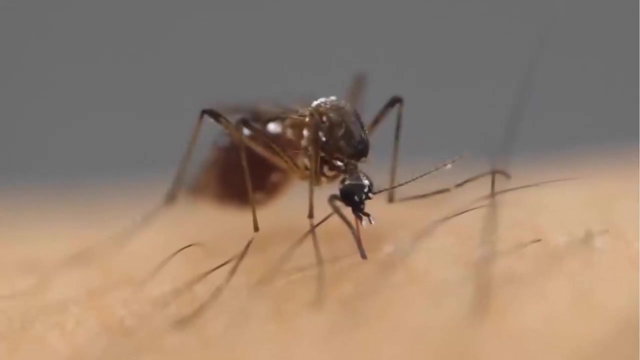 You are providing food to these mosquitos, So I'm a prey and the mosquito is the predator. No, you don't die when a mosquito bites you. This is another type of relationship. Mosquitos suck your blood to survive. 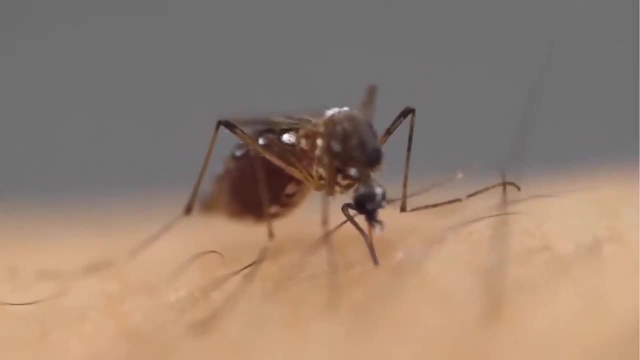 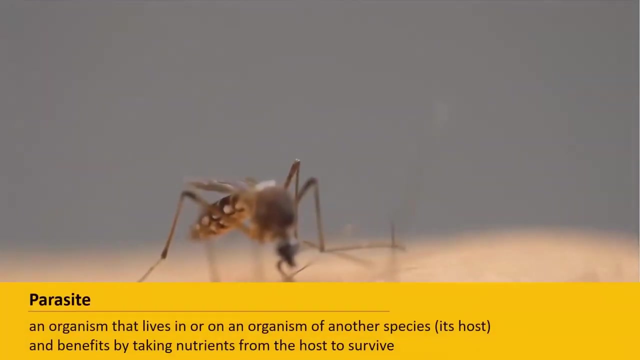 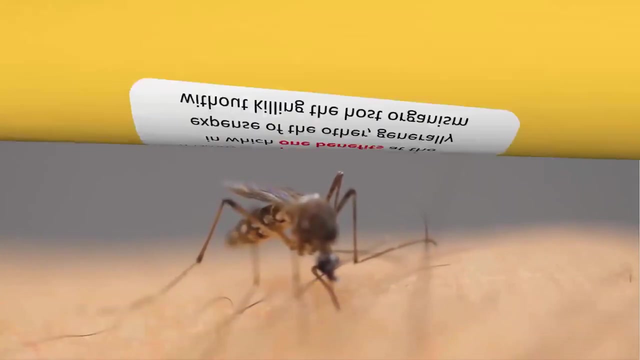 They also spread dangerous diseases like malaria and dengue. Such organisms are called parasites because it benefits from harming you. You are the host for these organisms, as they are feeding on you. This relationship between a parasite and its host is called parasitism. 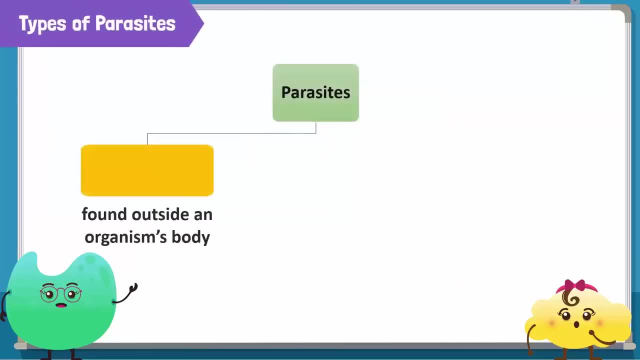 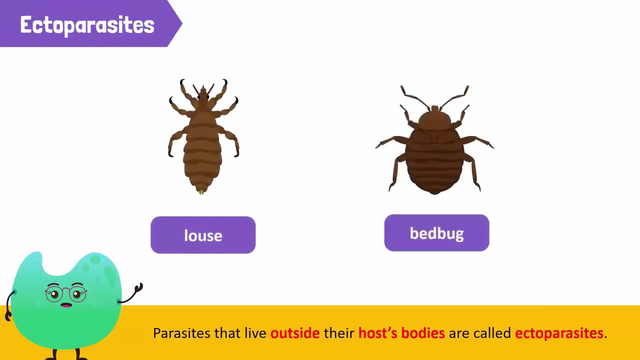 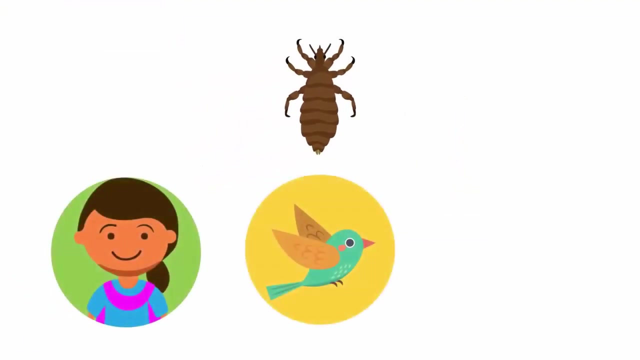 Parasites can be found both outside and inside an organism's body. Parasites that live outside their host bodies are called ectoparasites. Lice and bedbugs are examples of these parasites. Lice are parasites of humans, birds and many other mammals. 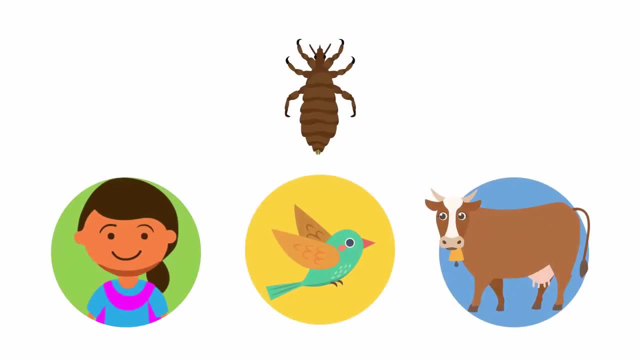 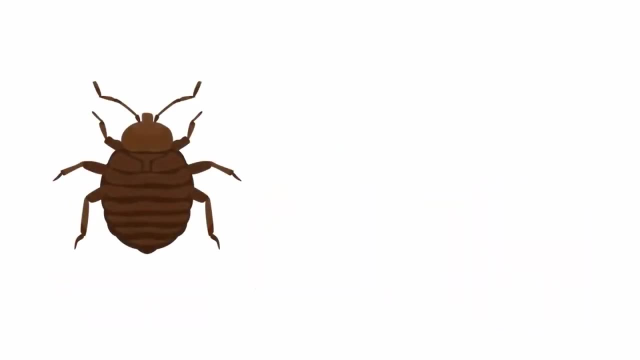 In humans, they're usually found in hair. They feed on their host's blood. Similarly, bedbugs also feed on humans' blood. They can bite humans on any part of their body. Their bites appear as red spots, which are often itchy. 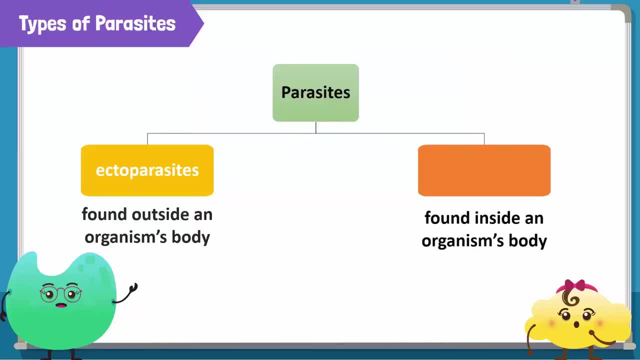 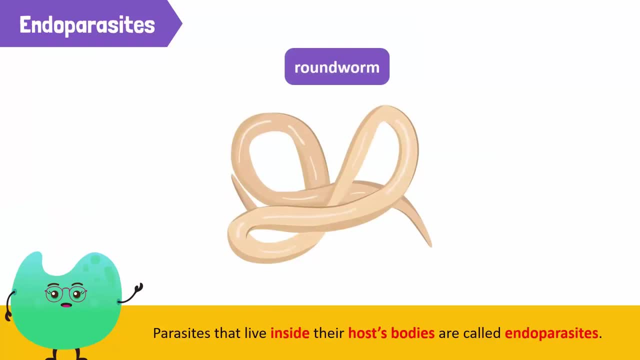 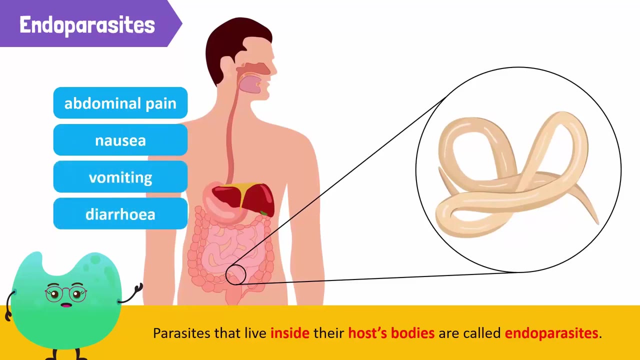 On the other hand, parasites that live inside their host's body are called endoparasites. An example of such parasites is the roundworm. They can be found in humans' intestines, which cause abdominal pain, nausea, vomiting, diarrhea and visible worms in stool. 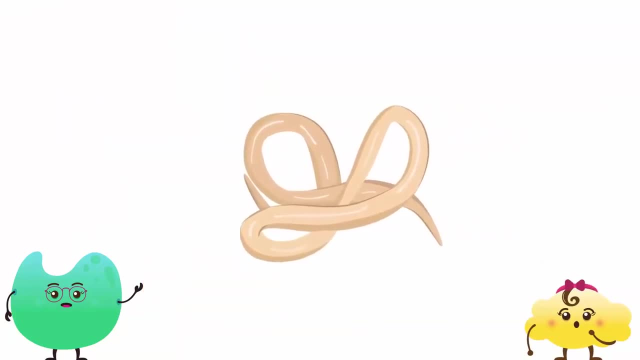 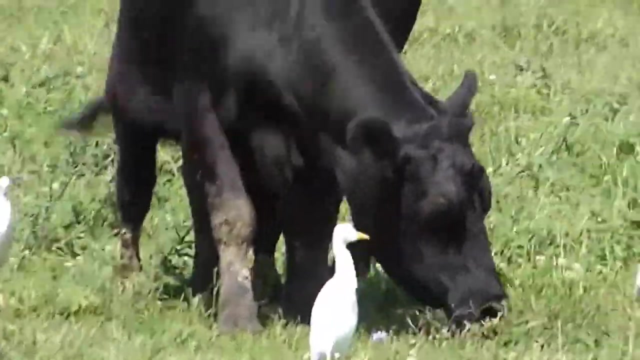 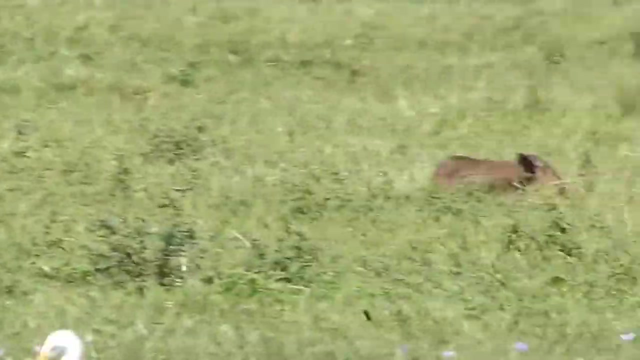 That is horrible? Yes, it is, But don't worry. There are some relationships that are of an advantage to both organisms. For example, look at that bird. It's continuously following that grazing cow. This bird is a cattle egret. It's quite common to find birds following cows, buffalos and zebras for food. 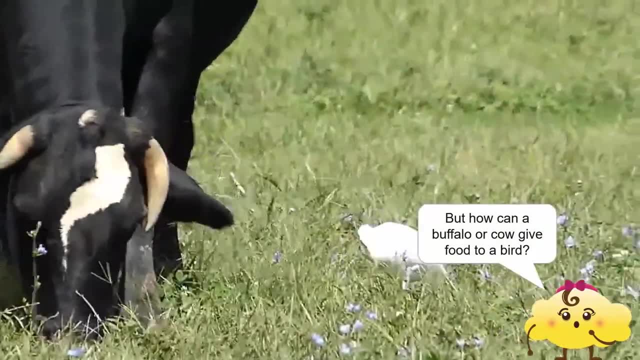 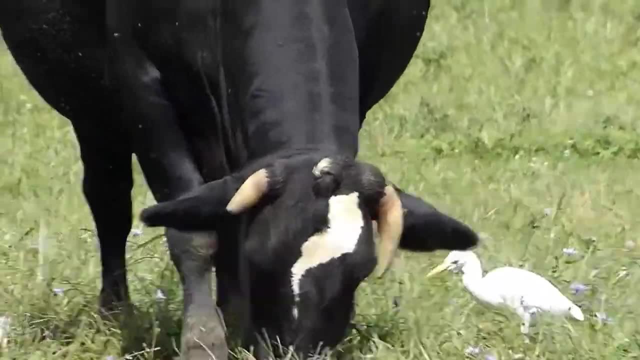 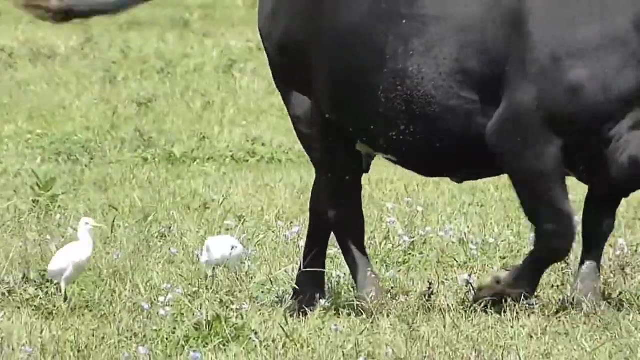 But how can a buffalo or cow give food to a bird? Birds follow the grazing animals and eat bugs and flies that tend to bother them. Sometimes they also eat parasites like lice and bugs on the animals' bodies. In this way, the birds get their food from these animals.